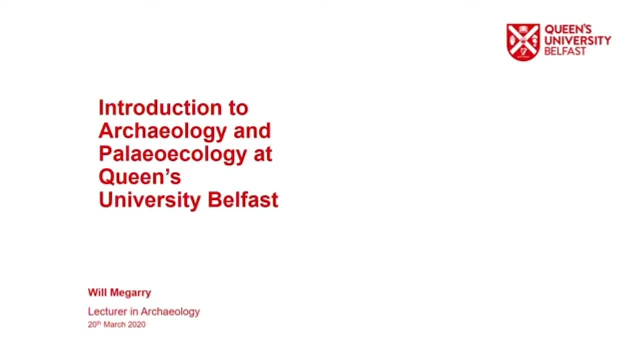 school of natural and built environment, and this includes the disciplines of geography, architecture planning and civil engineering. Archaeology and paleoecology is the smallest discipline and we have the smallest student cohort within the school, and most of our students take classes just within archaeology. Some then also take classes in geography and others depending. 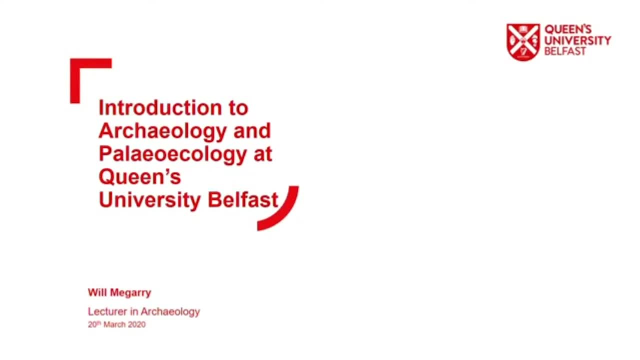 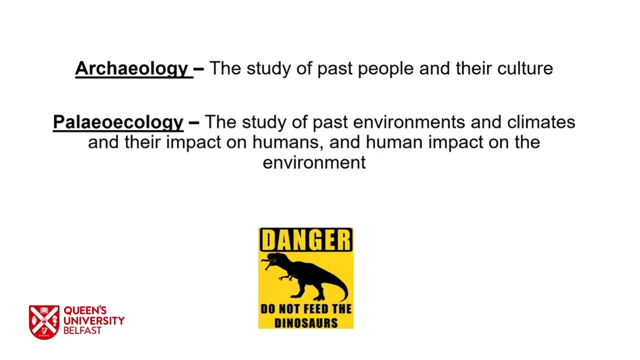 on the group program will also take classes in history and other subjects outside of the school. My name is Will McGarry and I'm a lecturer in archaeology and I've been in Queen's for about four years. So just before we get into the individual degree programs, just to go over a bit of definitions and 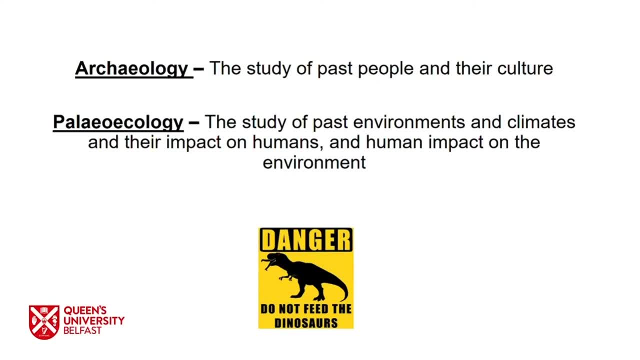 most of you will probably be familiar with what archaeology is. Archaeology is the study of past people and their culture. It is specifically the study of past people and their material culture. By material culture, I am referring to the things which people have made in the past and the things 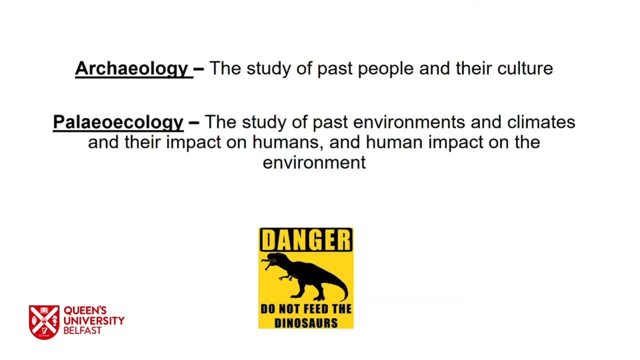 which are left behind by people from the past. This can involve everything, and from artifacts to skeletal remains And to all the way up to large landscape features like castles or earthworks. It can be distinguished from history because it's interested in the things rather than the record of the past. 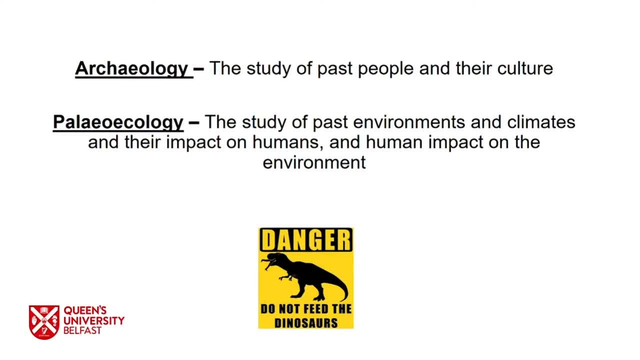 Paleoecology, then, on the other hand, is the study of past environments and climates and their impacts on humans, and then also, conversely, the impacts of humans on past climates and environments. It is not, I'm afraid, the study of dinosaurs. so if you are here looking to do a 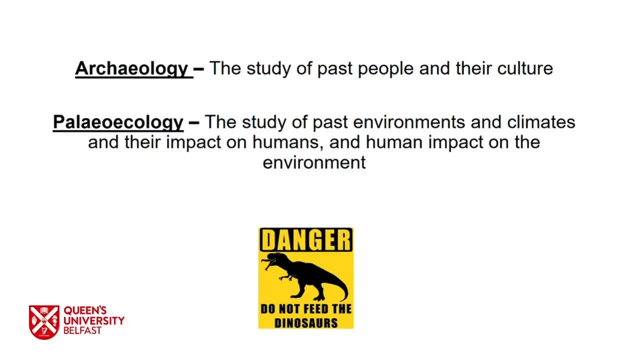 degree in paleontology, and this is perhaps not the quickest or most direct route to doing it, although we do have a lot of students who go on to study paleontology and as well. The combination of archaeology and paleoecology is really, really great, and especially when we think. 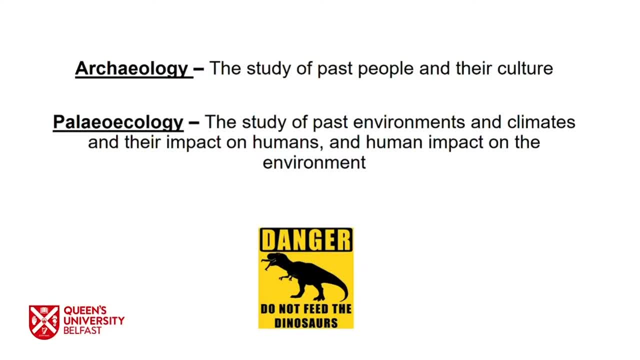 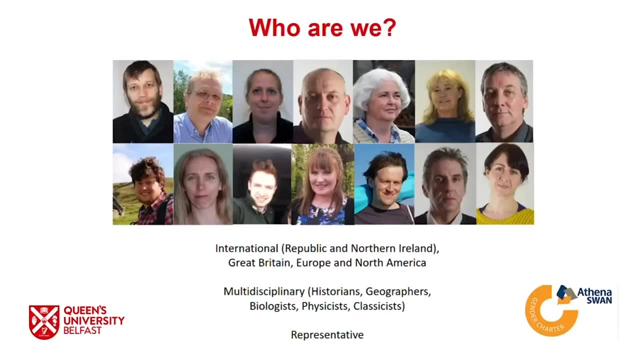 about many of the contemporary modern challenges we are facing, like climate change, which are really focused on human impacts on their climate and environment and how people in the past have learned to adapt and survive when these things change. So archaeology and paleoecology is both very, very interdisciplinary subjects. 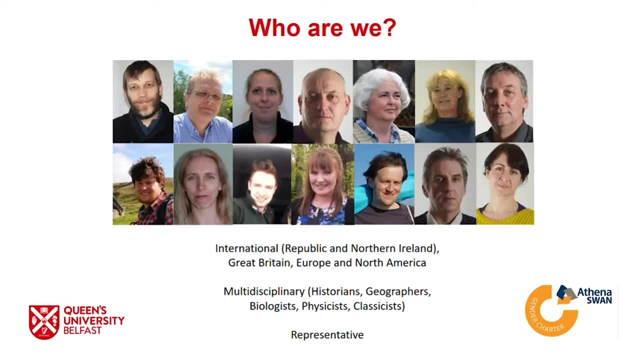 and that is very much reflected in the staff within the discipline. We come from a wide range of backgrounds, including history, geography, biology, physics and classics. We also come from all over the world, including many of us from the island of Ireland and Great Britain, and many from further afield, including Europe and North America. 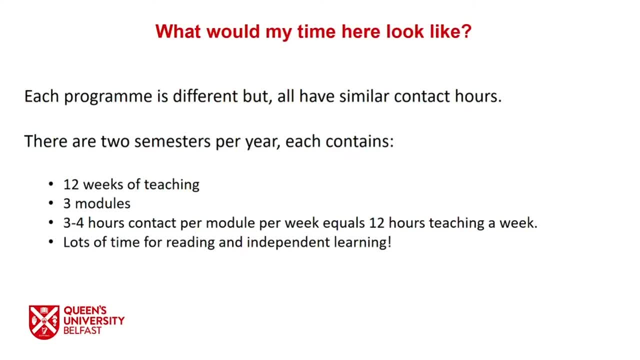 Now, you all probably have offers for different degree programs, and no two programs are exactly alike, but there are some similarities, and so what I want to go over today is just some basic questions about what your time here will look like, and one of the most common questions we get. 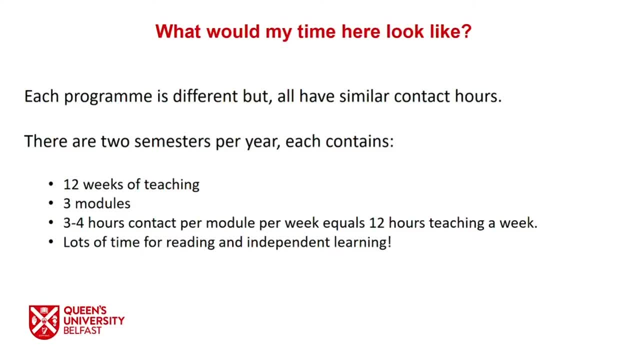 is how much time am I actually going to spend in university, and this can be quite different from your experience of school and because you'll find there's an awful lot less direct contact hours in university than there was during school. So the academic year is broken up into two semesters. 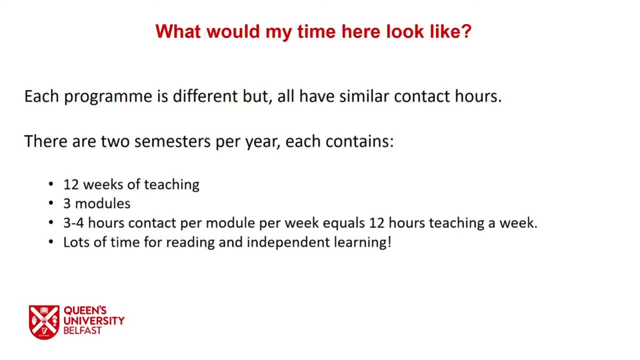 and each semester will contain 12 formal weeks of teaching. Within each semester you will be expected to do three modules, and each module will have a certain number of credits. Each module will contain between three and four hours contact, so those are either lectures or tutorials, and so if you do a little bit of math, you'll work out that that probably means you'll be 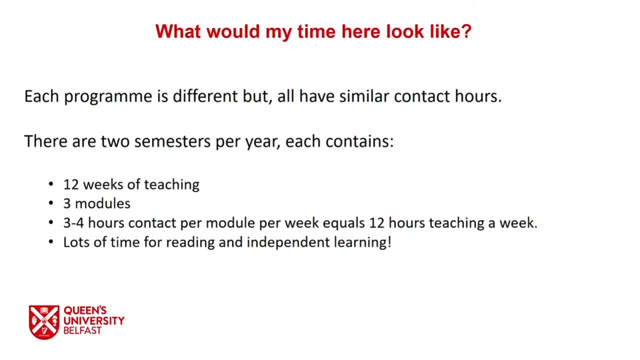 a maximum of about 12 hours a week in either classrooms or lecture theatres during semester time. So what that means is there's quite a lot of time when you're not actually being taught, and the thing about university is this is an opportunity for you guys to learn. 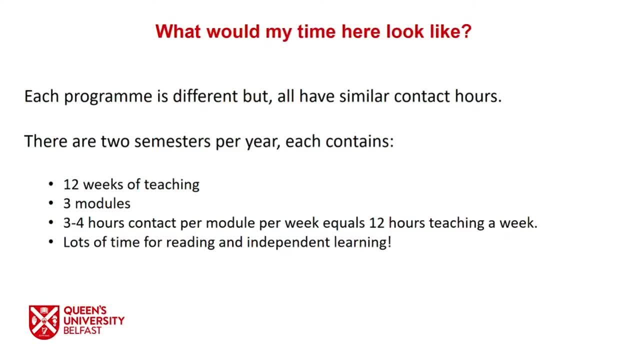 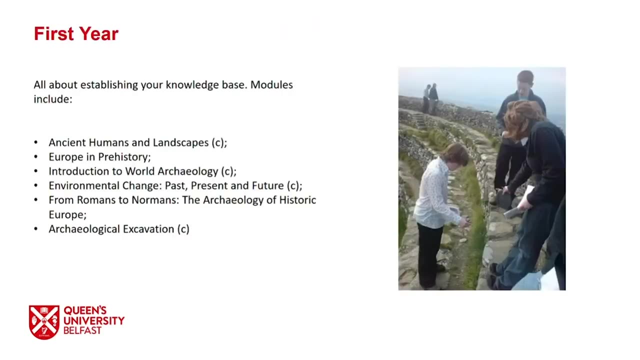 how to learn independently, and an awful lot of that time is going to be spent reading books and articles or spending time in the library. Some of it will be spent doing group work or working with your individual tutors on different things. The first year of all our degree programmes focuses on level one modules, and these are modules which are based on establishing your knowledge base in the subject of archaeology and paleoecology. 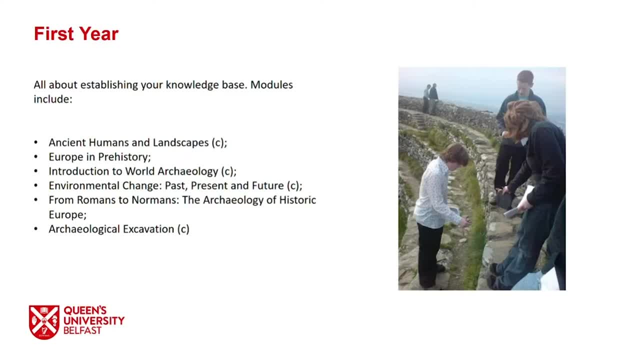 So they are really assuming that people are coming in with very little knowledge of these two disciplines and giving you a good foundation upon which you can learn in subsequent years. So, for example, these include modules on introduction to world archaeology, which takes a look at the main cultures and material cultures from around the world. 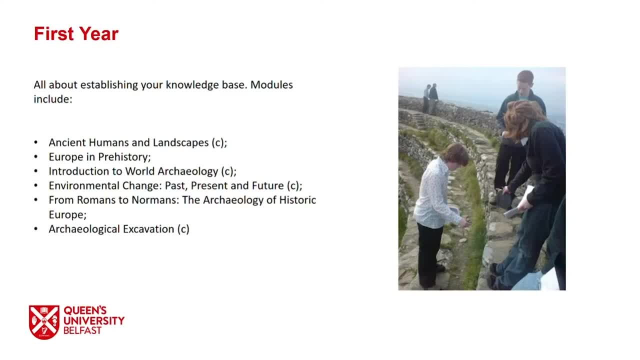 They can include modules on environmental change- past, present and future, or thinking about how ancient humans lived within their landscapes. There is also, for most people, a compulsory excavation module, which happens in June every year, after a term is finished, and that is a practical archaeology module where you will go out on an excavation with members of 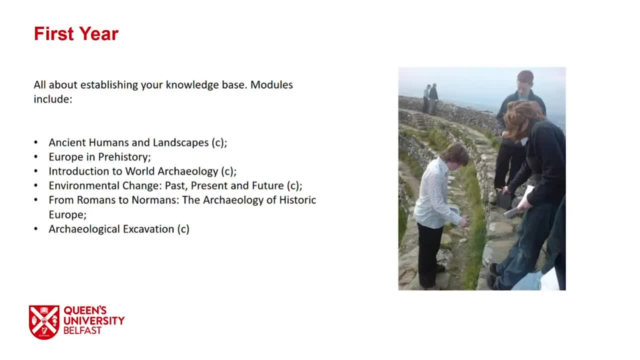 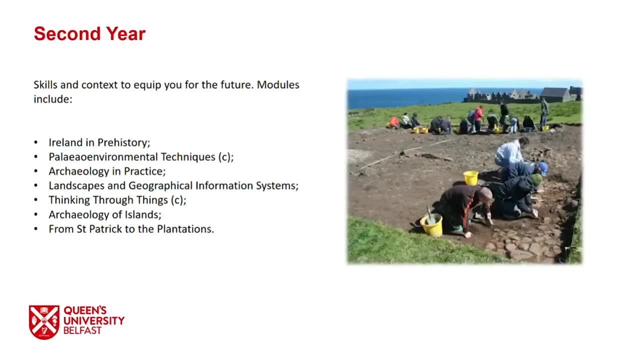 staff from Queen's University and you will learn how to put your archaeological skills in practice in the field By the time you get to second year. it is really focused on giving you guys the skills and what you will need to equip you for your future. So there are a lot of techniques. 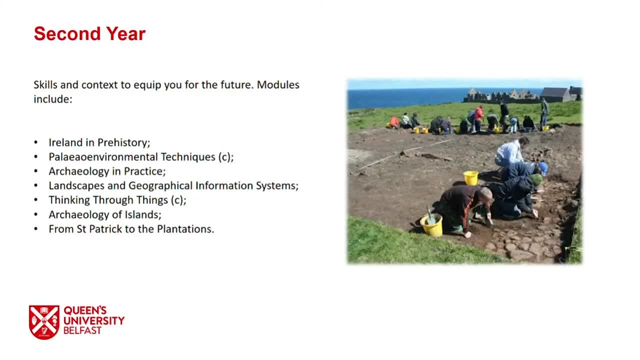 based modules in this year, including paleoenvironmental techniques, which are the techniques and skills you would use to understand past landscapes and past landscape change. There's a module, archaeology in practice, which is very much focused on the practical elements of archaeological excavation and associated things. 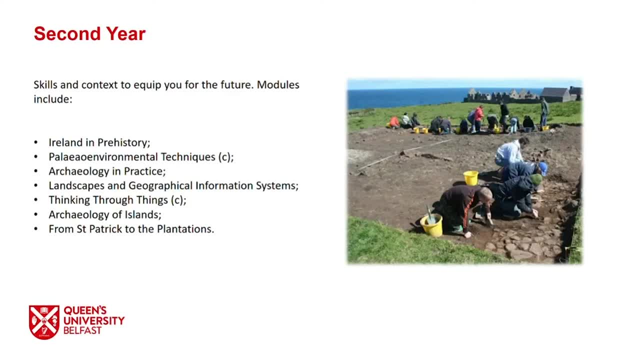 like survey and making maps. There is a theoretical course called thinking through things which goes through an awful lot of the theory about how we think about things and how we interpret things within archaeology and that is a preparatory module for the dissertation module which you will do at level three. There are also other optional courses and including the 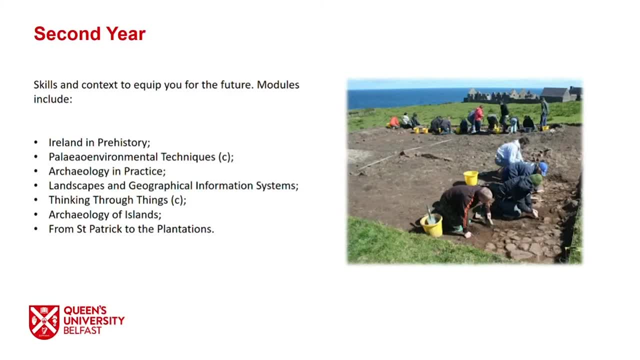 archaeology of islands, which is our field trip module, where we go away for a week as a class, usually in semester two, and modules on historic Ireland or St Patrick At the end of second year. a lot of you will have the opportunity if you want to take it. 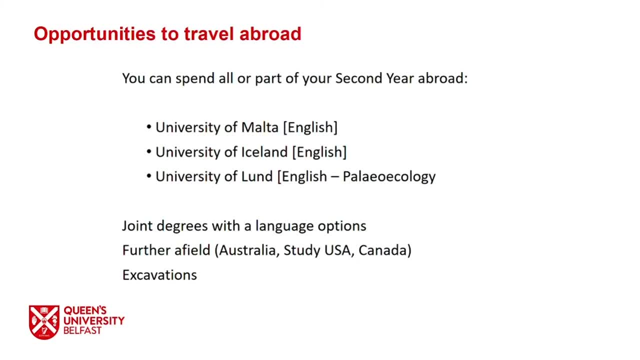 to travel abroad now. some of you will be involved in language programs where you're doing archaeology with a language, and this will be expected of you at this time. For those of you who aren't part of a language program, there are still plenty of opportunities to travel. this includes opportunities. 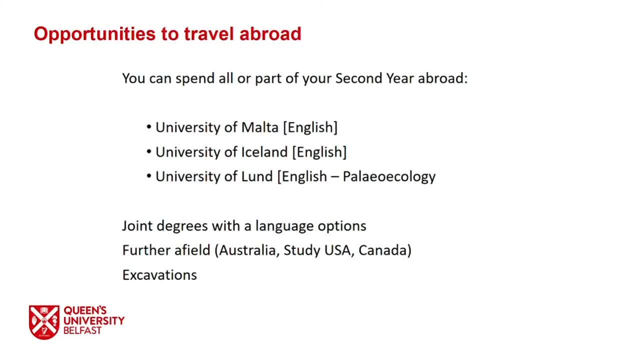 to go to, in your next year or so, Universities and institutions which Queen's has formal agreements with, including the University of Malta and Iceland, and And also opportunities to go further afield, if you wish, through programs the university offer Including study USA or opportunities to go to Canada. 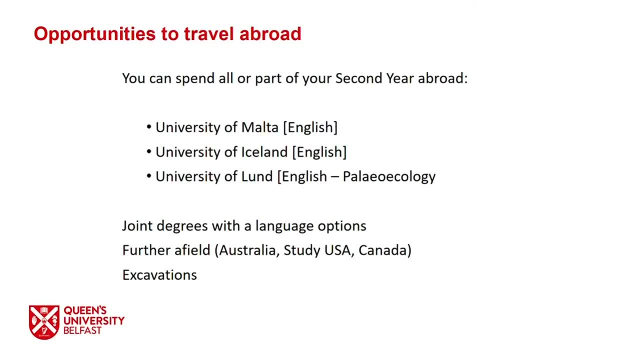 We have a relationship with several Canadian universities and our students. every year a number of them will go and take opportunities of those. There's also usually the opportunity at the end of second year to get involved in other excavations, either commercial excavations or excavations Run by members of staff. So whereas at the end of first year excavation will be a training excavation, at the end of second year 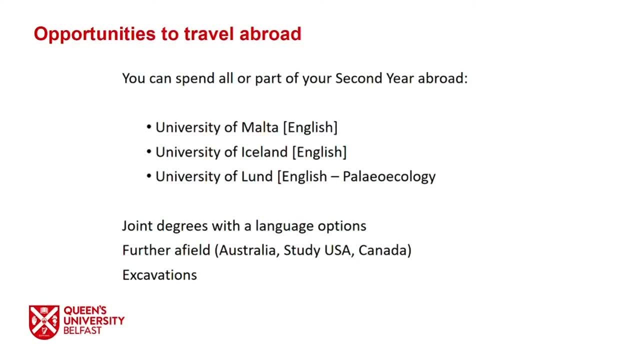 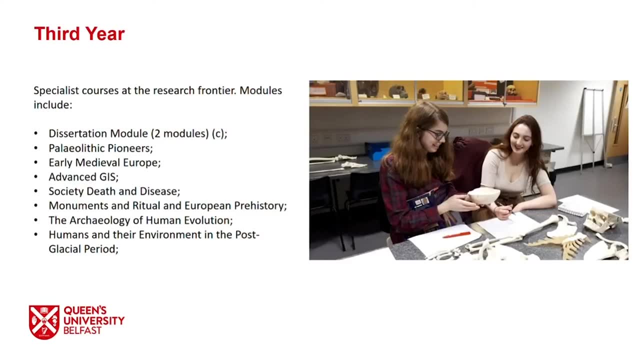 Most of you will have the opportunity to get involved in actual excavations and to apply those skills practically in the field. Third year, then, is often the most intense year for our students, because this is the year where you will Do a dissertation module. a dissertation module is double-weighted. 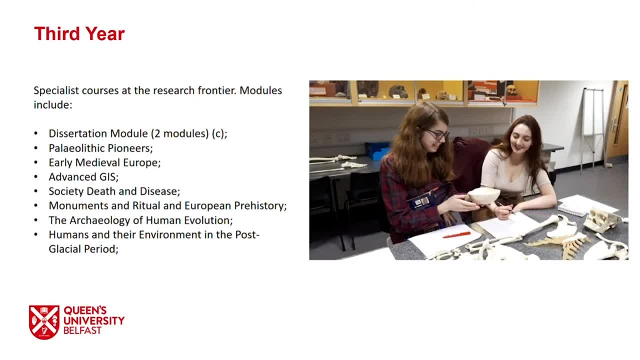 It runs throughout the two semesters and this is when you will work with a supervisor to create a piece of individual research, usually about 12,000 words for the words long. You will also get the opportunity in third year to do more specialist courses, So this is often where our students will develop. 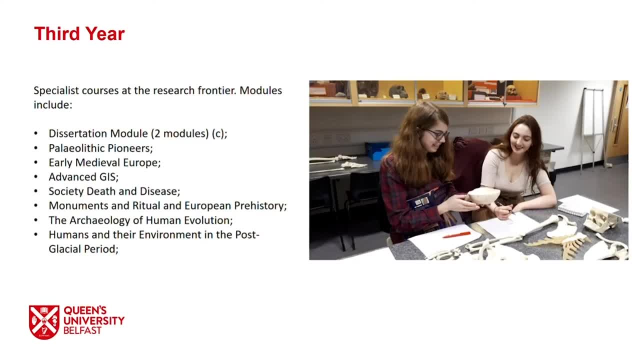 More specialist skills in areas like mapping or survey, and the society death and disease module, which focuses on the practical skills, And of osteoarchaeology, or some of the more paleoecological Specialist courses we offer. like humans and their environments in the post-glacial period. 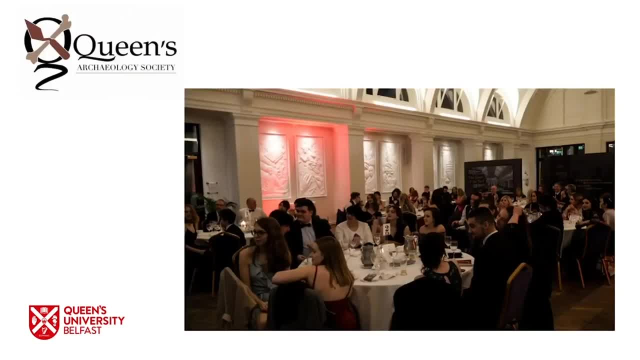 Of course, your time in the university is not just about formal education. It's not just about spending time in modules. It's also a great opportunity for you to make friends and get involved in other things, and we have a very active Archaeology Society in Queens which organizes trips abroad and lectures and then also organizes the annual 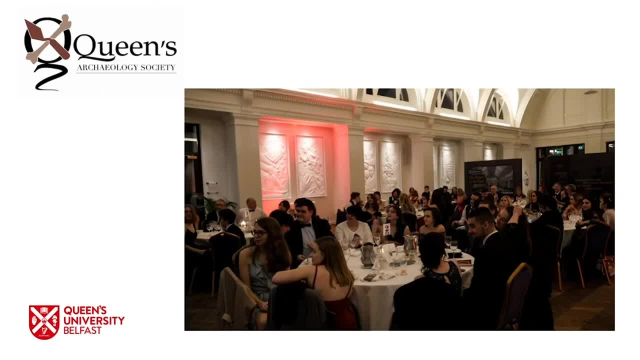 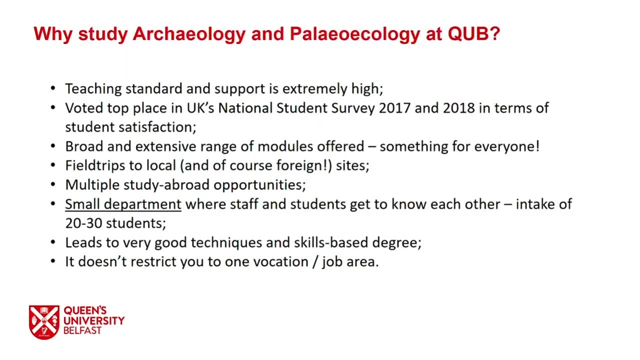 Formal every year, which is usually attended by most staff and students studying archaeology. So why study archaeology and paleoecology at QUB? Well, I mean, obviously I think it's great, right, but it's not just me. our students actually think it's great as well. 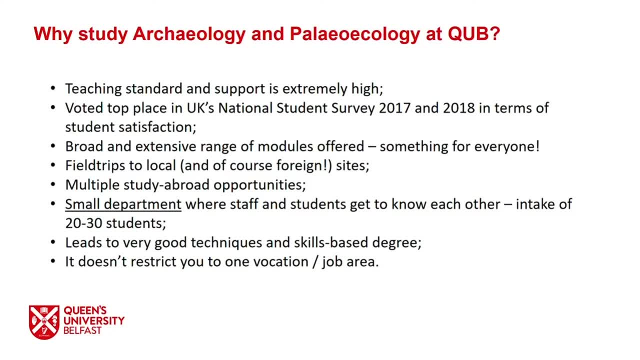 We've been voted top place in the UK's National Student Survey in 2017 and in 2018 in terms of student satisfaction, And one of the reasons we think this is the case is that our teaching standard is very, very high. We're very fortunate in being quite a small discipline. 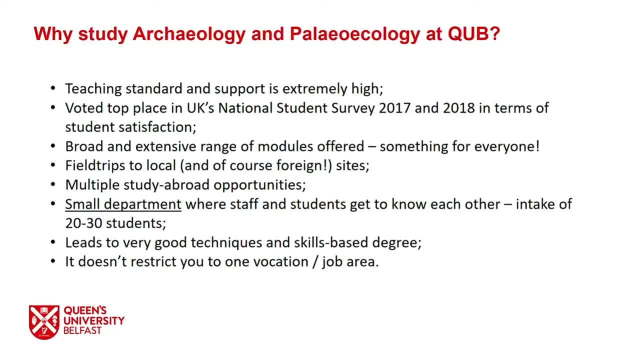 It will be very rare that within Archaeology you will ever be in a class with more than about 30 people in it, and certainly by the time you get to second And third year, the numbers are normally even lower than that- still, usually between 15 or 20. 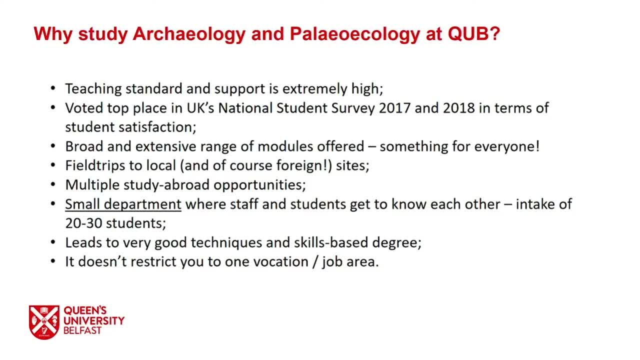 We offer quite a broad and extensive range of modules, and not just within archaeology, But there's also the opportunity to take modules outside of archaeology. So many of our students take modules in anthropology, geography and history and archaeology. Archaeology is a very, very practical 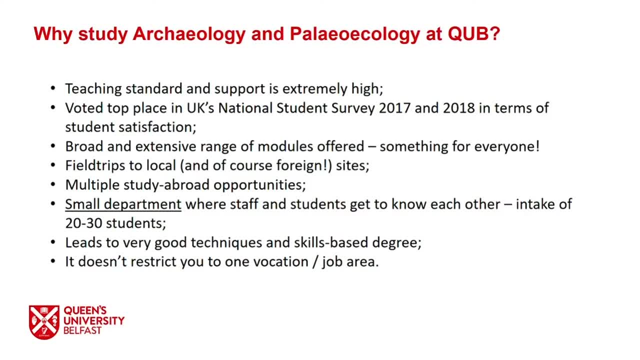 based module and we do an awful lot of field trips as part of your modules, and so they might be Longer term residential field trips over about a week or short-term weekend trips to sites around the island of Ireland And, but one of the key things that we like to get out and about, we like to go and do and see things. 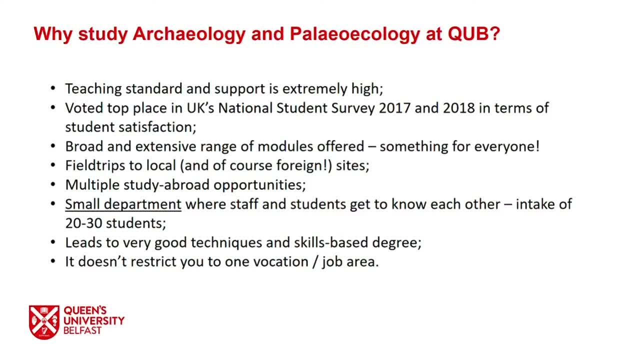 in the field. In fact, paleoecology is very similar to this and we will have you out on bogs taking quarrying samples and we will then be taking those samples back into the labs and showing you guys how to analyze them and look at them and 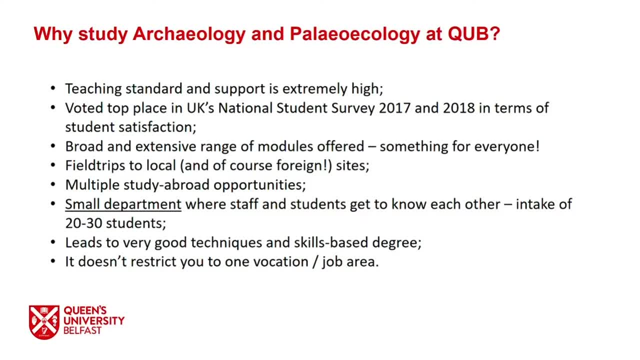 in the lab. Archaeology and paleoecology are both also really good skills based degrees, So our students go on to work in all sorts of areas. many of them, rather unsurprisingly, go on to become Archaeologists. some of the go on to use their paleoecological skills in climate change research. 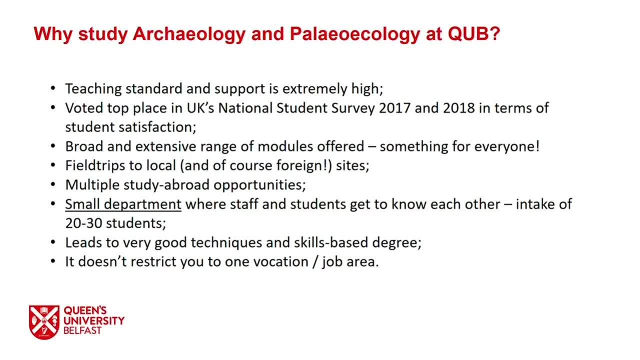 Many of them go on to work in organizations like the LPC, Yes or the ordnance survey. others go on to work in museums and some people go on to work in non heritage based sectors entirely. Some people go and do teaching. one of the great things about archaeology is that it really encourages. 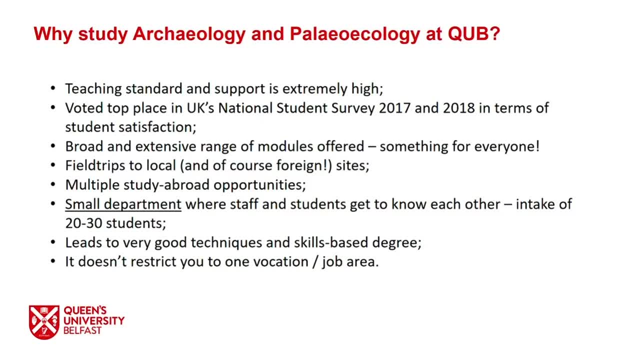 Independent learning, and it encourages a set of skills that are highly transferable and to just about anything that you might want to do, So it doesn't restrict you into one vocation or job area. It gives you an awful lot of opportunities from a practical perspective and 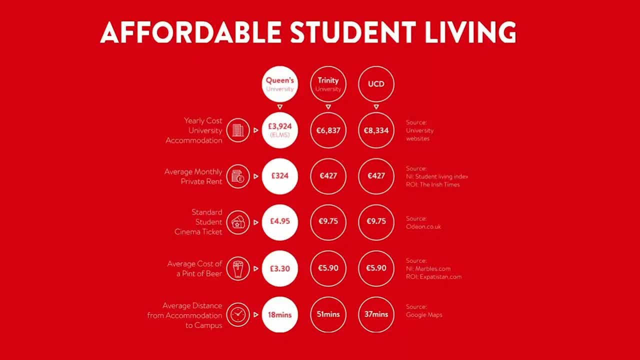 Belfast is also just a really, really good, fun, safe place to live and it is Substantially cheaper than other places on the island of Ireland. So if you're thinking about coming up from the south- and it is a lot cheaper to live in than Dublin- your monthly rent will be substantially smaller and your 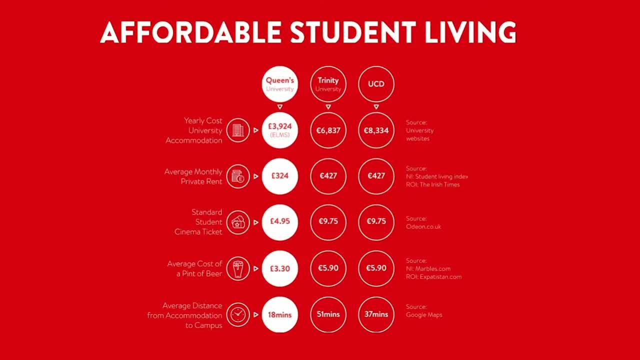 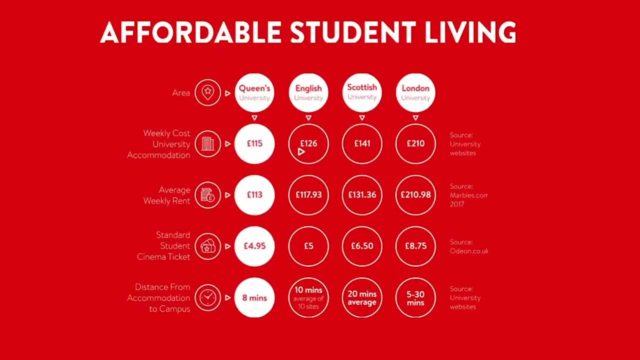 entertainment and Socializing costs will be an awful lot smaller as well, and Belfast as a city is incredibly walkable and safe, If you're thinking about coming from wider GB, and Queens and Northern Ireland is also much, much cheaper than just about any other part and of the United Kingdom. and these are all. 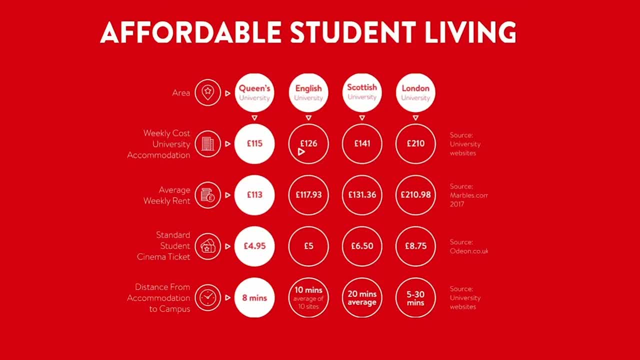 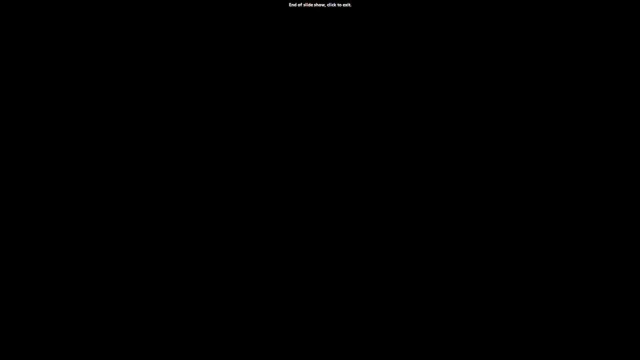 Serious considerations to think about and during your time here. So I hope that's been a useful overview of the different programs which we offer and please do feel free to email me or any other member staff if you have any specific questions about the programs and 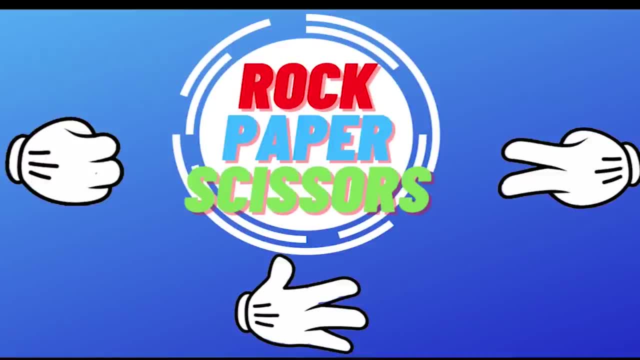 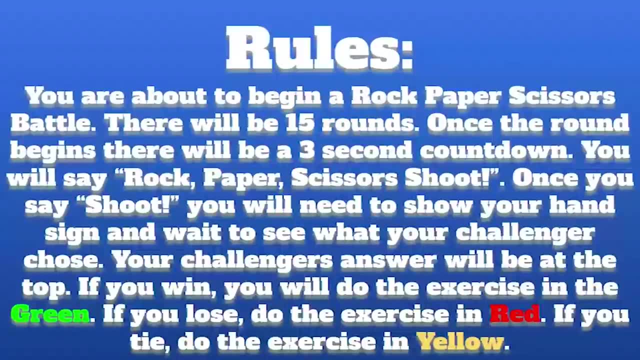 You are about to begin a rock-paper-scissors battle. There will be 15 rounds. Once the round begins, there will be a three-second countdown. You will say: rock paper scissors, shoot. Once you say shoot, you will need to show your hand, sign and wait to see what your challenger has. 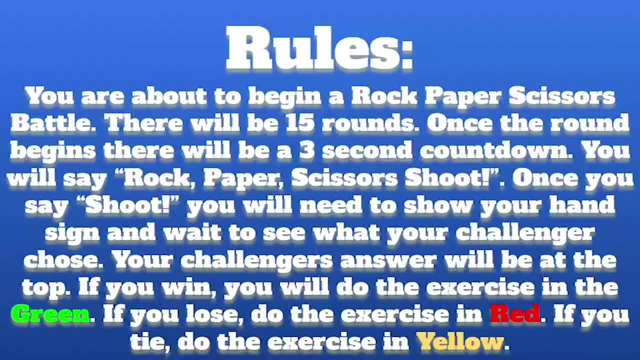 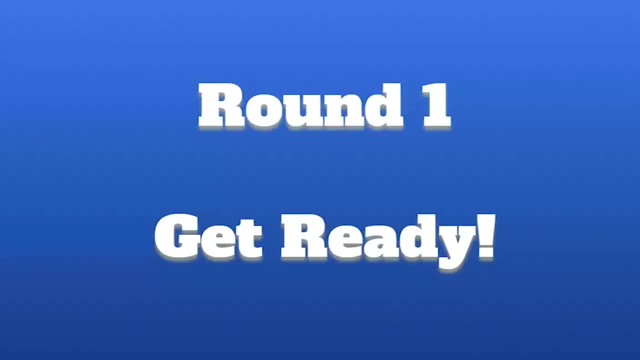 chosen. Your challenger's answer will be at the top of the screen. If you win, you will do the exercise in green, If you lose, do the exercise in red, And if you tie, do the exercise in yellow. Round one: 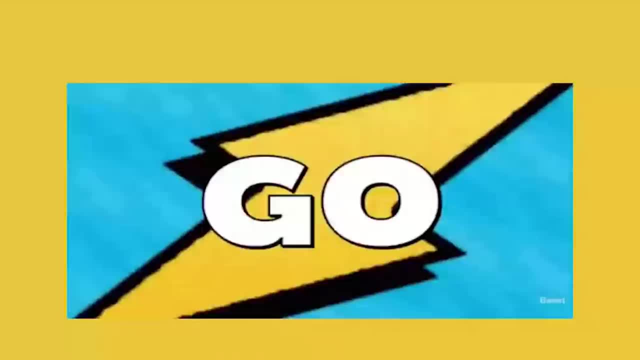 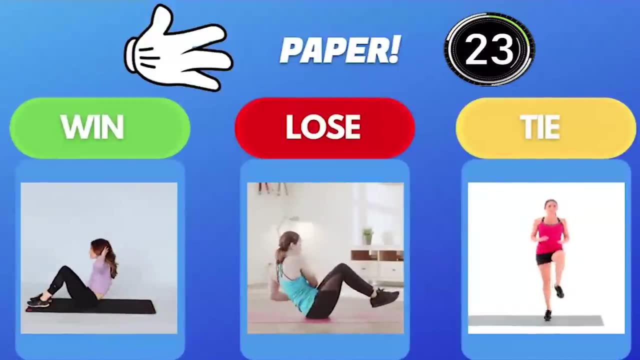